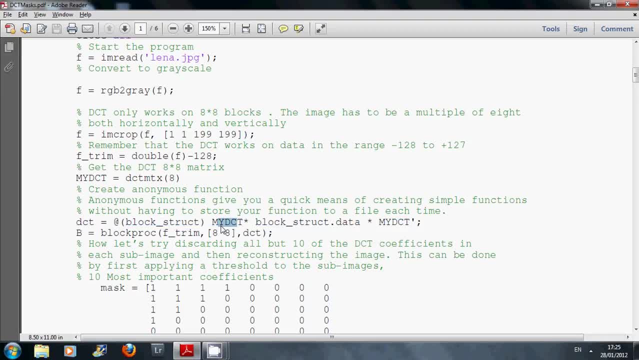 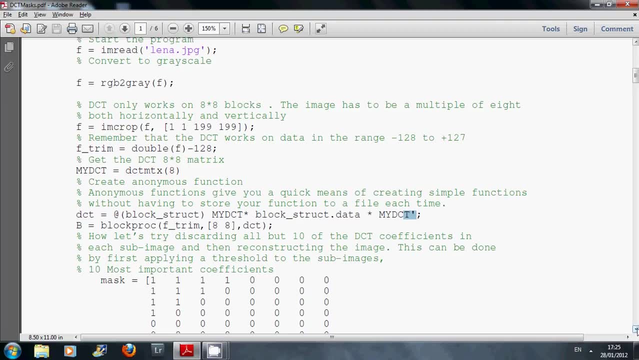 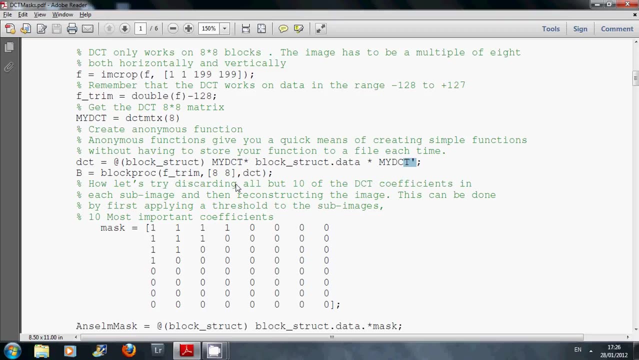 So my DCT is my anonymous function. My DCT comma is the transpose and the block structure dot data. So I've explained before. So here we go, Your block processing. What are your block processing? The original function: Well, it was modified to 128.. 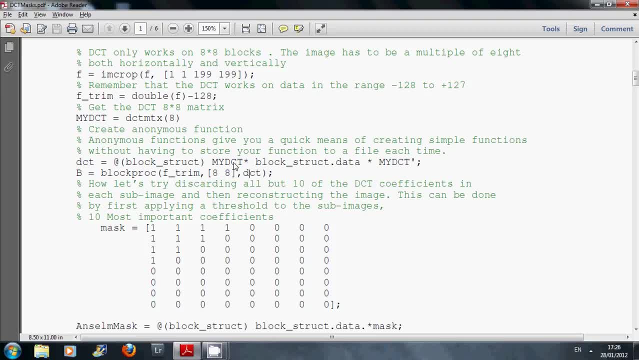 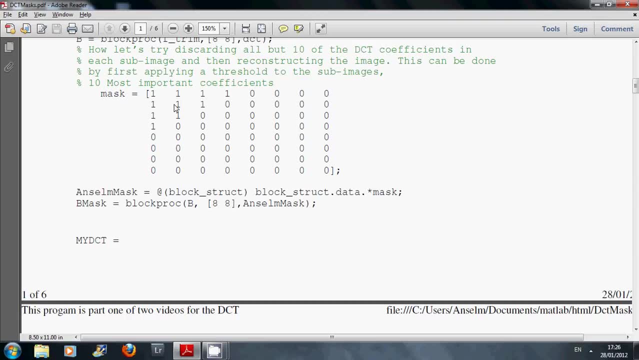 In 8 by 8 blocks, And the function that we're applying is the one that you defined here, my DCT. So you've done all of that. And then what did this mask do here? This mask here will keep the 10.. 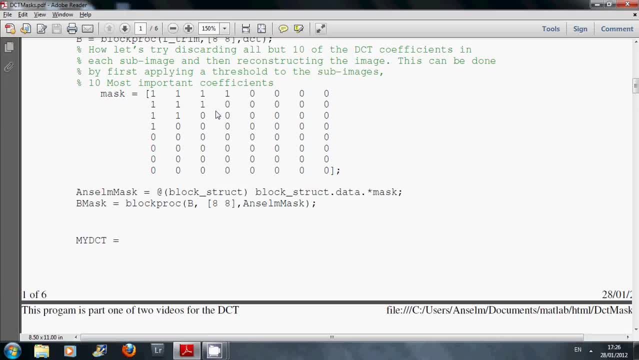 Well, I was going to say the 10 lowest AC, but actually it's the DC and the lowest 9.. Okay, So I ran this anonymous function here, I defined it on this line And I ran it there. So what that does is it goes through 8 by 8 blocks. 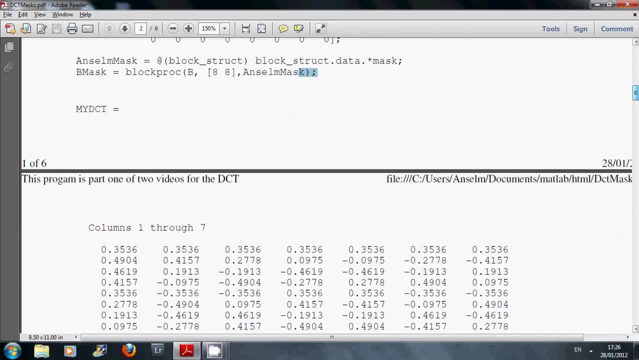 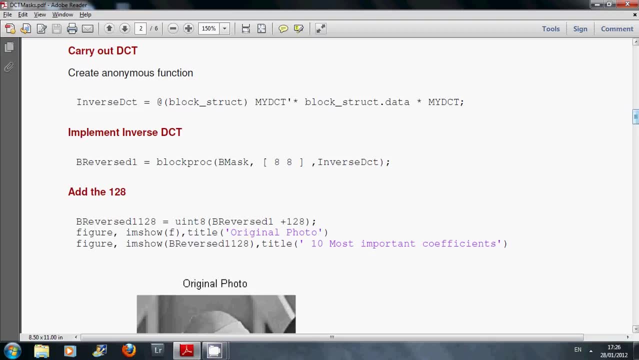 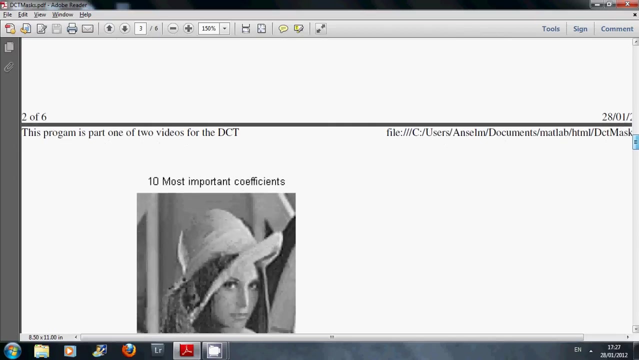 and it's keeping the 10 lowest coefficients. There's my DCT MTX function. So then I inverse my data. Okay, Defined my inverse function, Ran it And added on the 128.. There's the original in grayscale And there's the. 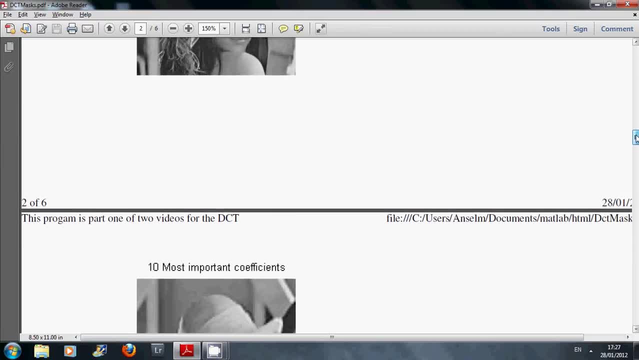 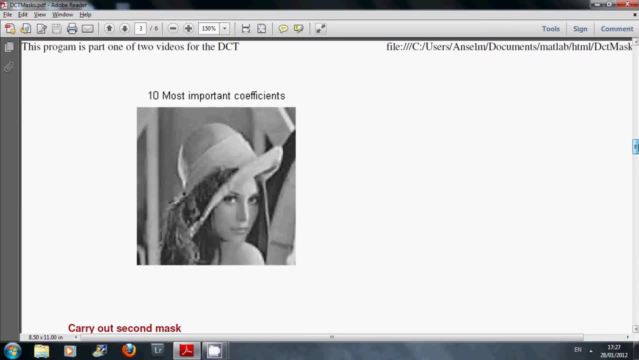 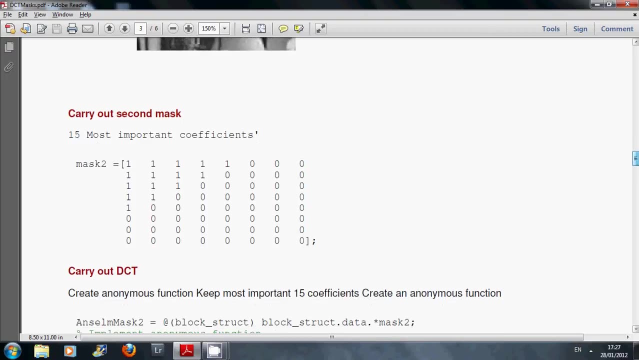 Now it's a bit hard to see, But you can kind of see here that You know it's a reasonable representation, It's not too bad. So I repeated this again, And this time I upped the number of The coefficients. 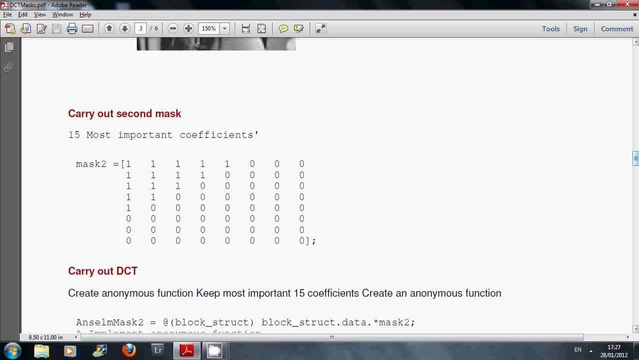 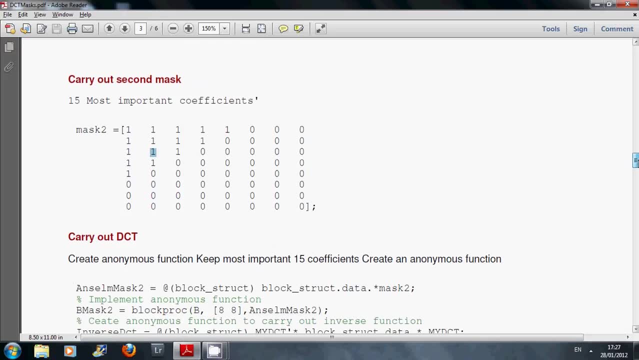 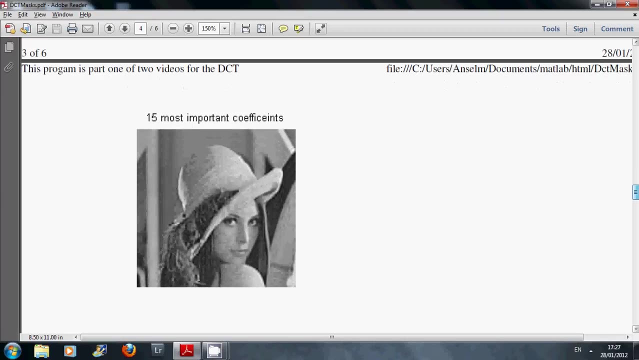 I upped the number of frequencies, I upped the number of the AC And this time I was keeping the 15 most important. Same functions, again, Anonymous, that I defined above. And there's the 15 most important coefficients. And when you run this, 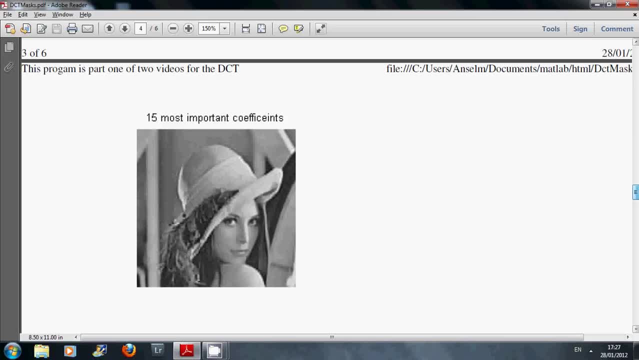 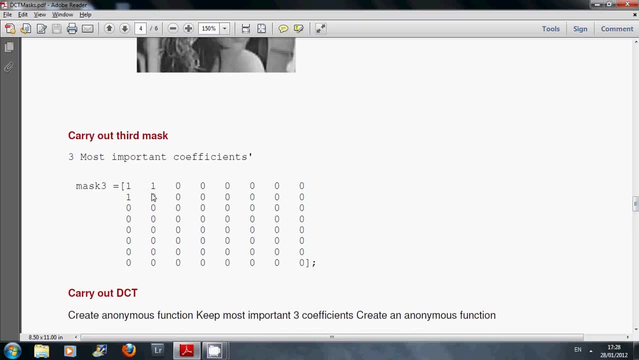 you would expect and hope that the 15 mask would be better than the 10 mask. I did it again And this time I'm only keeping three terms. I'm keeping the DC and the two lowest AC. There's the image there.